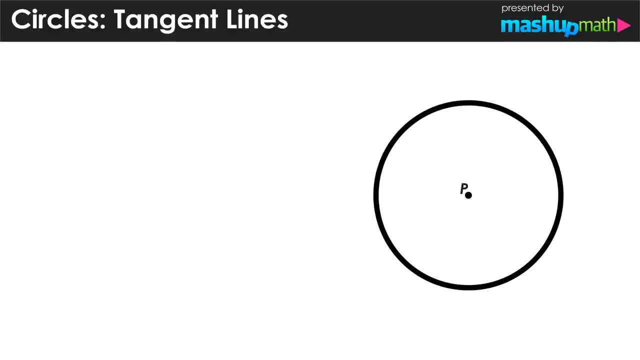 the relationship between circles and tangent lines. So let's start with the question: what is a tangent line to a circle? So let's take a look at a circle with a center at point P And let's also imagine another point on the circle and we'll call that point T. 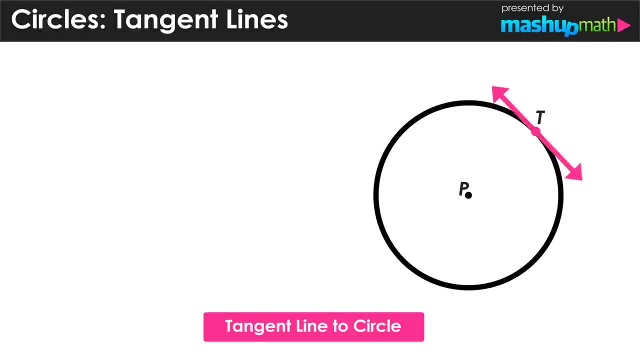 A tangent line to a circle is a line that intersects the circle at exactly one point, in this case our point T. Now if we construct a line that connects that center point P with that point T, on the outside of the circle we would be constructing a radius and we can call that line R. So PT is a radius. 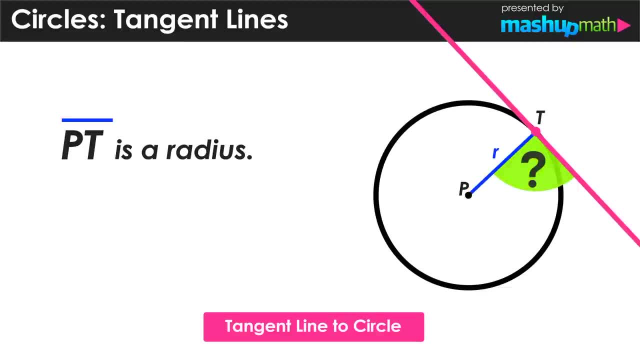 of circle P And if we look at the angle created by the radius and the tangent line, we should see that this appears to be a right angle, measuring 90 degrees, And this is the case with tangent lines and circles, And we can say that a tangent line is perpendicular to a circle's radius. 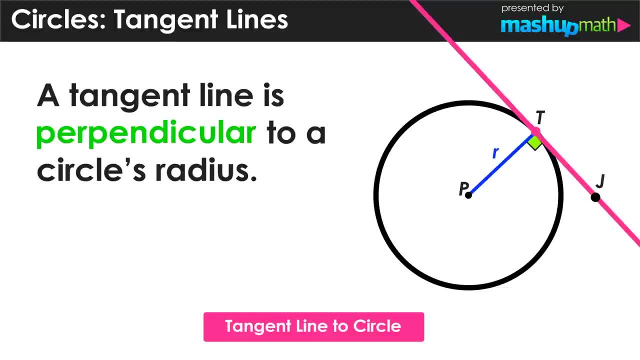 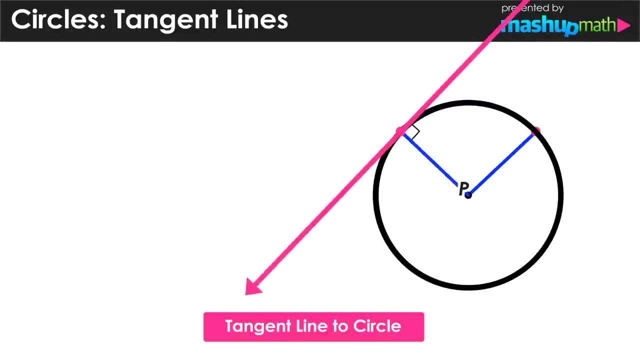 So if we add another point on the tangent line, point J, we can conclude that angle PTJ has a measure of 90 degrees And this perpendicular relationship between a circle's radius and a tangent line applies to every circle in any occasion. So the key concepts to understand here is that a tangent line intersects a circle at exactly one. 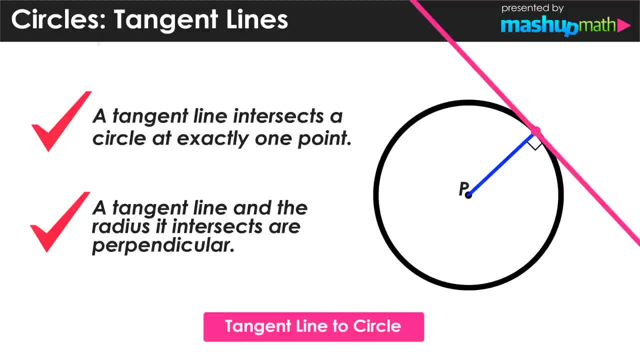 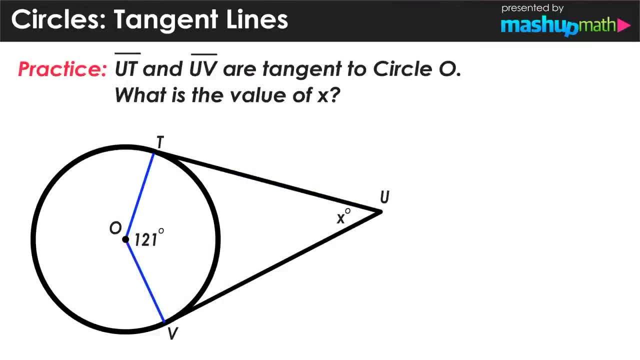 point, and that a tangent line and the radius it intersects are perpendicular. Haha, cool. So now let's go ahead and apply our understanding of tangent lines and circles to a practice problem. In this case, we have line segmenting. We have line segment UT and line segment UV, both being tangent to circle O, and we're 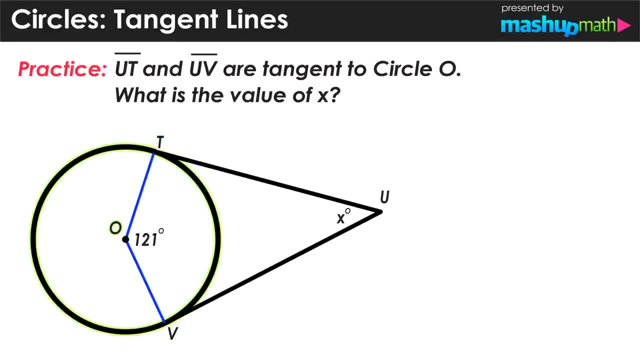 looking to find the value of X shown on the diagram. So notice that lines UT and UV are line segments. however, they are still tangent to circle O, which means that they will still hold the same properties of tangent lines, even though they are not infinite lines. 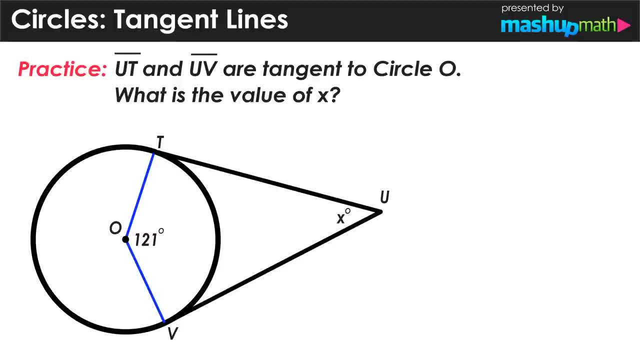 And we should also note that we know that angle O has a value of 120 degrees And that angle U is the value of X that we are looking to find Now. we know that UT and UV are tangent lines to circle O, and we know that a tangent line 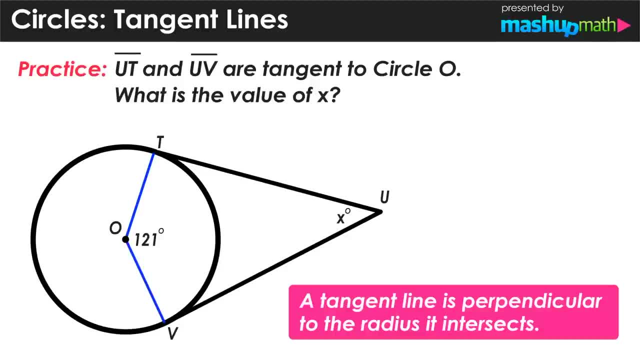 is perpendicular to the radius it intersects, So we can conclude that angles T and V are right angles and have measures of 90 degrees. We should also notice that we are dealing with a quadrilateral here in this diagram, And we know that the sum of the interior angles in any quadrilateral is always equal to 360. 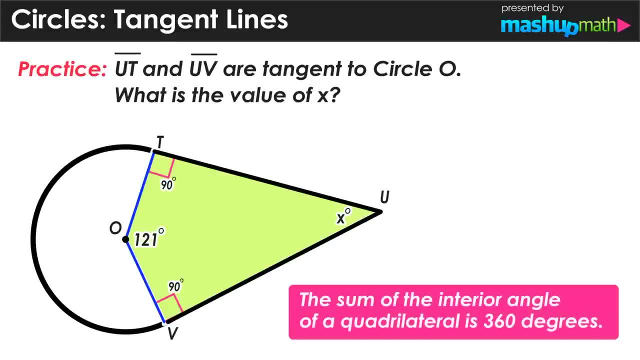 degrees. So if we take these four angle measures and add them together, their sum will equal 360.. And we can use this fact to find the value of X, 121 plus 60.. That's 360.. That's 90.. 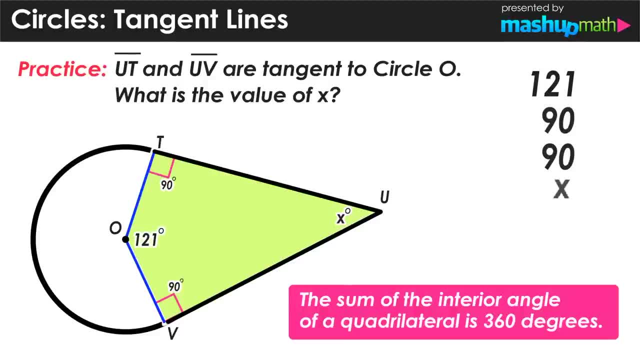 Plus 90.. Plus whatever X is is going to equal 360.. And now we can just use some basic algebra to isolate the value of X and find out its value. In this case, adding the three angles that we do know gives a value of 301.. 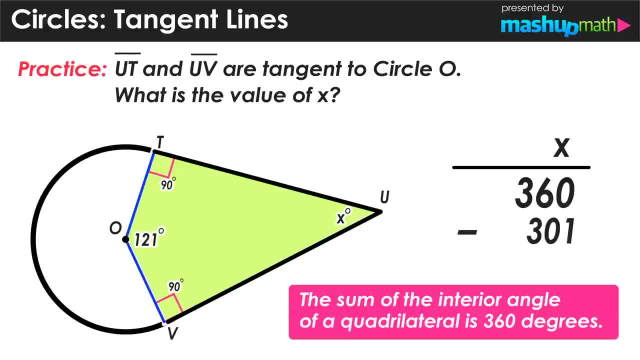 Subtracting 301 from 360 results in 59, which is the value of X, And we can conclude that angle U is 59 degrees. So now that you understand the properties of tangent lines and circles and have got some more experience applying those relationships to practice problems like this one, you can 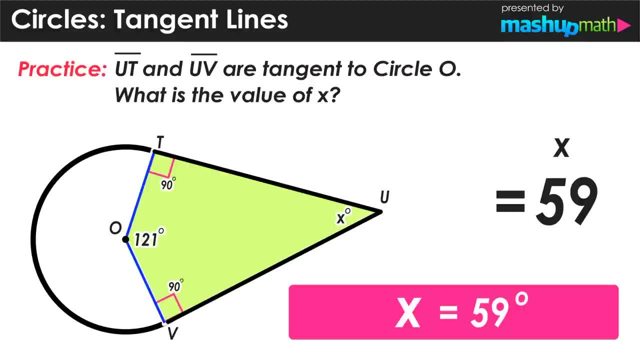 continue to apply your skills and understanding to future problems. So thank you again for stopping by everyone, and I'll catch you soon. Cool, All right. So that's it for this lesson. Thank you again for stopping by. I hope you found it helpful. 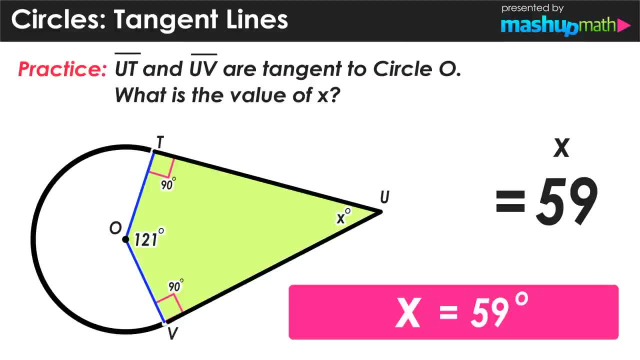 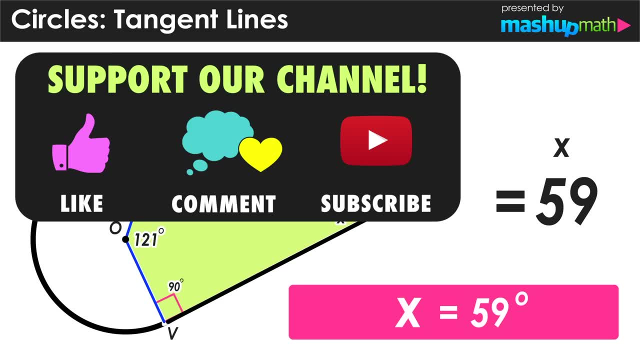 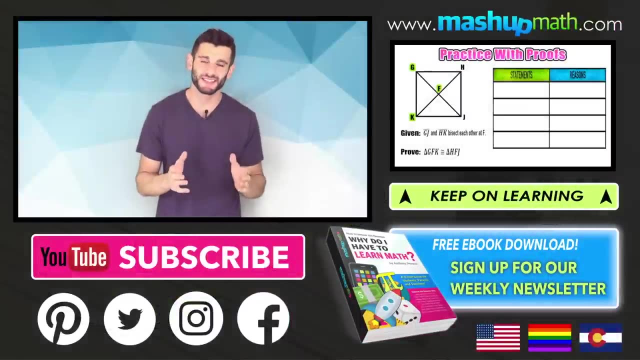